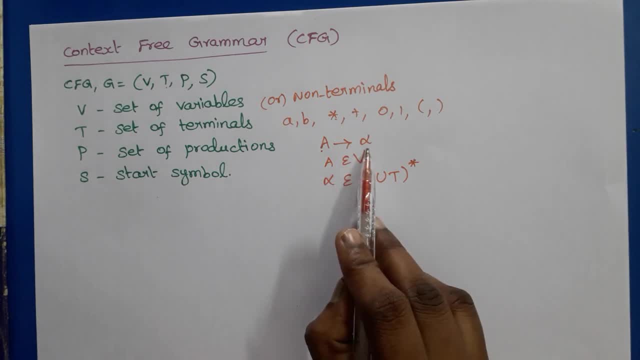 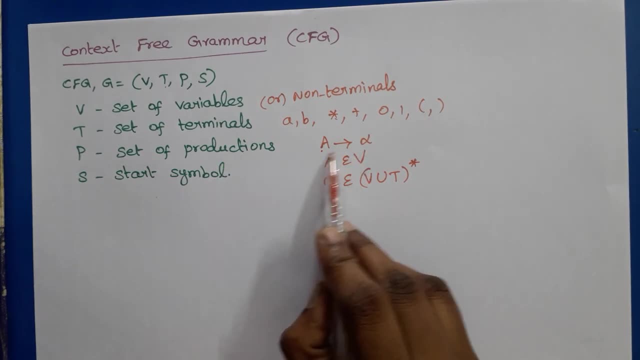 production symbol, a variable production symbol, followed by any number of variables and terminals. so this is a form of writing production. here, this symbol, this variable, represents head of the production and this one represents body of the production. the left side of left hand side of arrow mark production symbol is a head of the production and right hand side of the production. 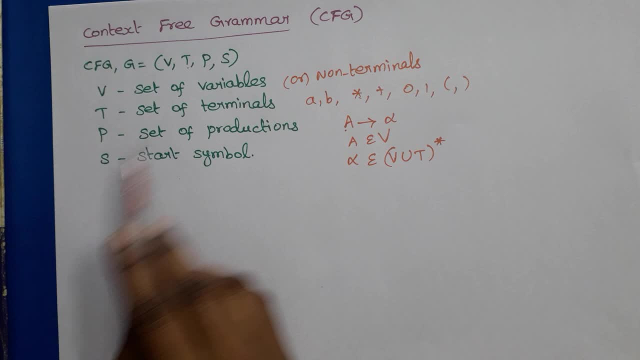 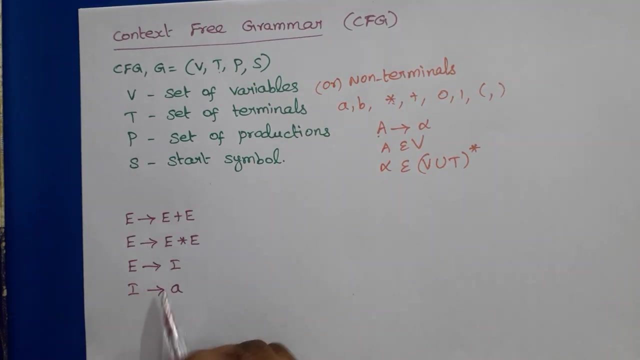 symbol is a body of the production and the last component is yes, yes, represents start symbol of the grammar. so this is normally the head of the first production. this is start symbol of the grammar. so, for example, consider these set of productions where you, this production, this grammar has four productions. so first one is e, tends to e plus e. 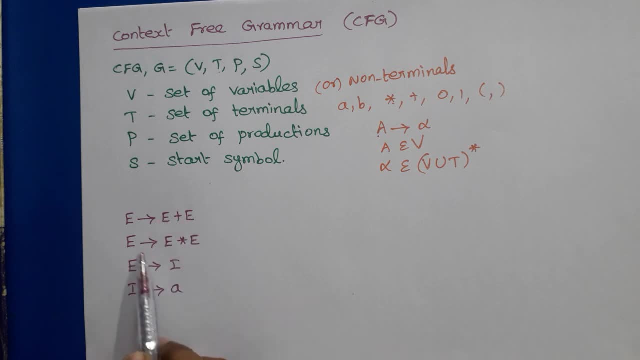 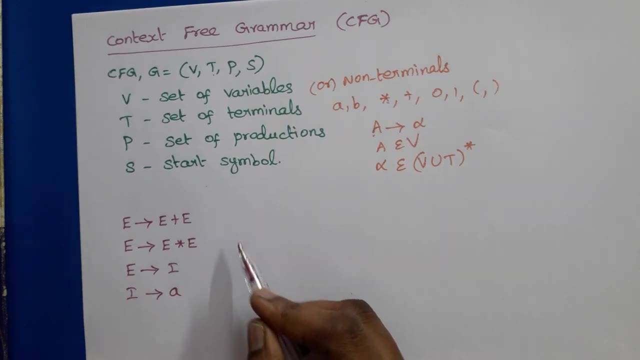 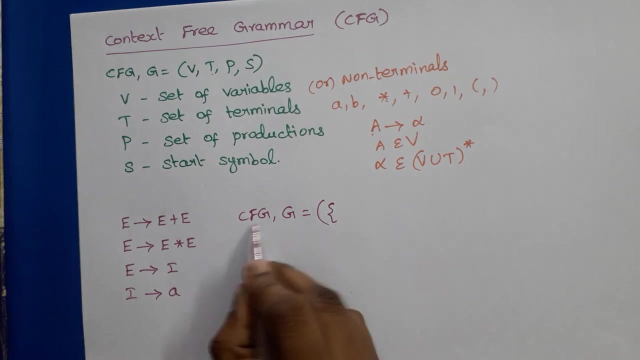 an arithmetic addition expression and e can be e, star, e, e tends to i and this i is a. i tends to a, so the grammar can be written. the four-triple notation can be written as: cfg g is equal to set of variables, so what are the variables used in this? 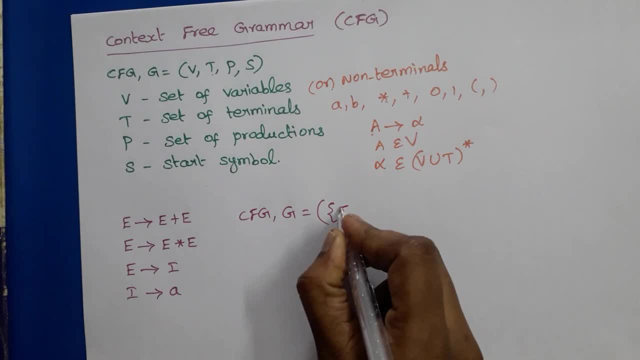 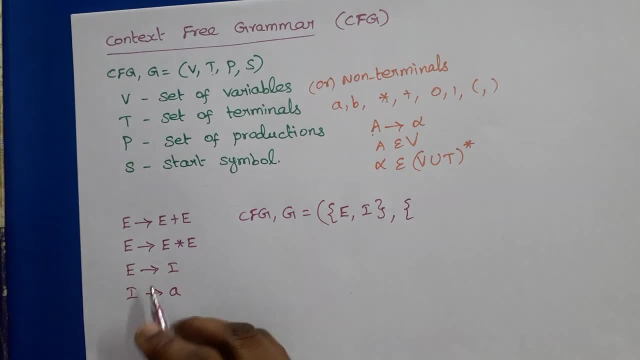 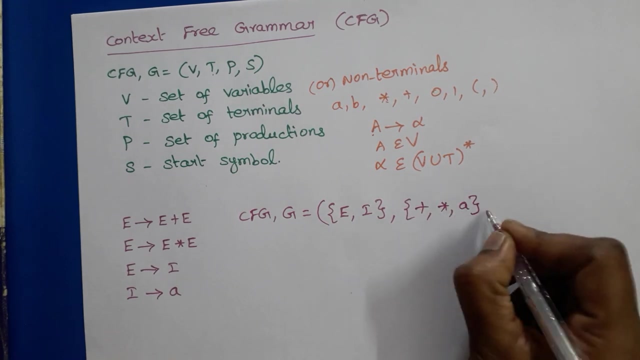 grammar: e, e and i right, so e, i. these are normally represented by the capital letters, so e, i and the set of terminal symbols used in this grammar are plus star and a. plus star, a and set of productions- p. set of productions. we have already written, so this is: 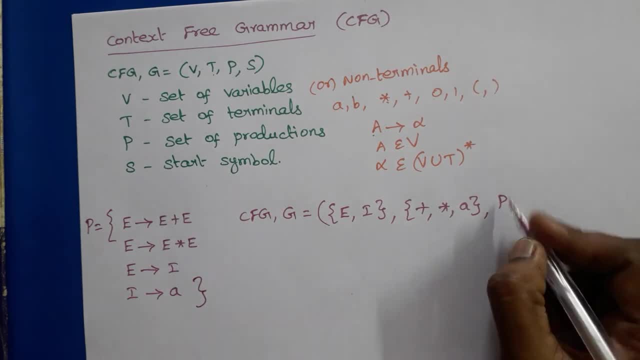 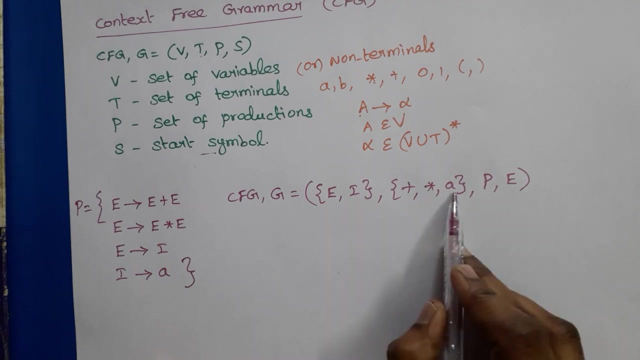 this: these are the set of four productions for this particular grammar- then the start symbol of the grammar- normally the symbol of the grammar is head of the first production, so e. so this grammar has a set of variables, ei set of terminals plus star a, and set of productions. 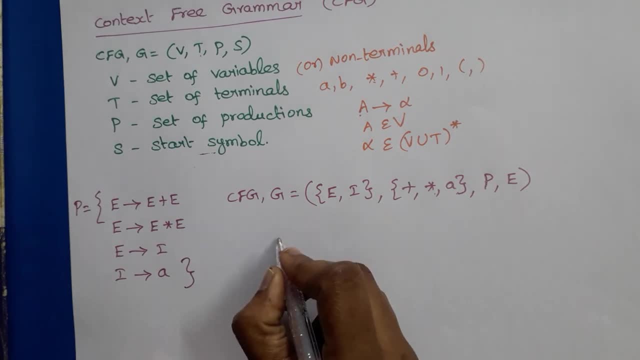 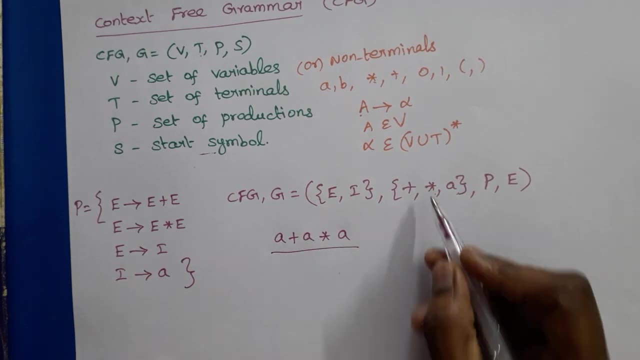 and e. now we can derive a string from this grammar: a plus a star a. this is the input string and the input string consists of all terminal symbols right: a plus a star a. so we can derive this string from the start symbol of the grammar. this is called as derivation, so derivation means 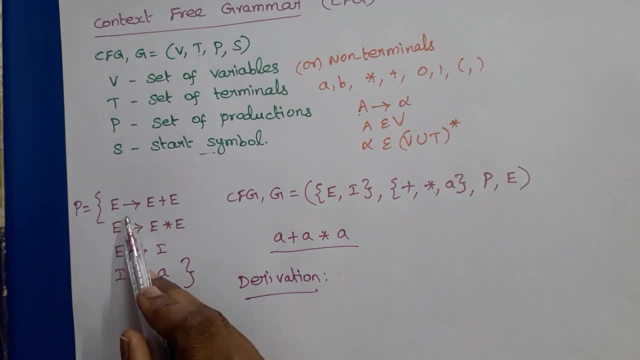 we can derive the input string from the start symbol of the grammar by one or more steps. in one or more steps by replacing head of the production by body of the productions right. so derivation means we can derive the string. we can expand the string from the start symbol of the grammar by replacing head of the production. 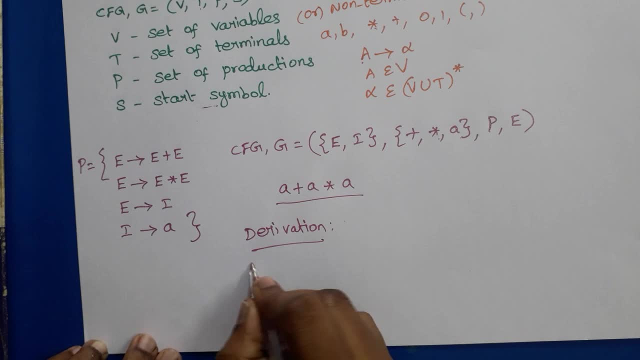 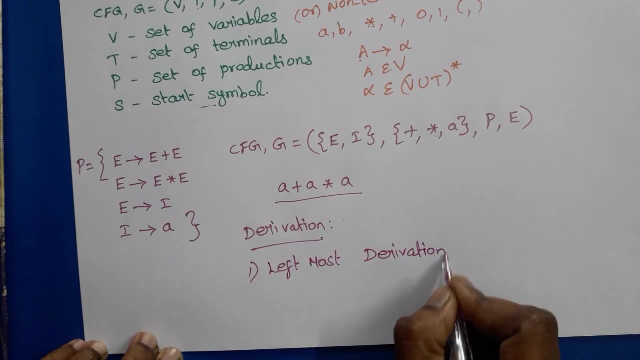 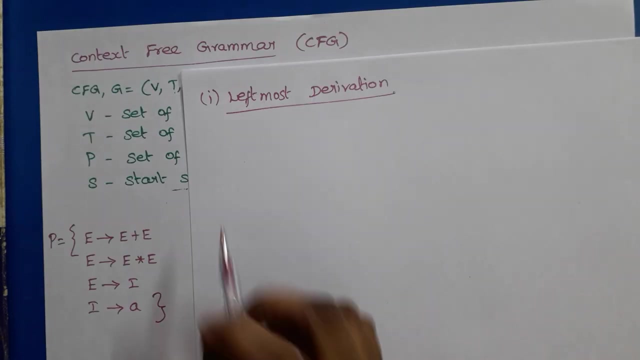 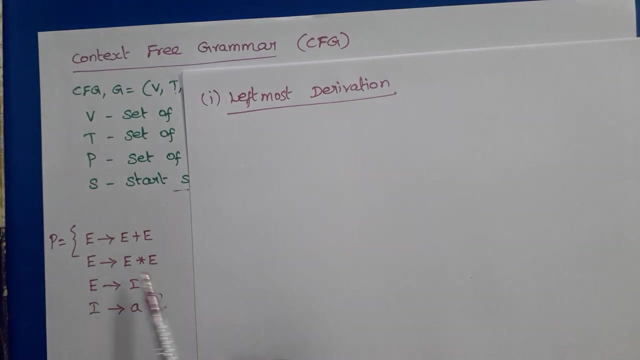 by its body of the productions. and there are two kinds of derivations. one is leftmost derivation and another one is rightmost derivation. so in leftmost derivation, at each step we replace the leftmost variable by one of its production bodies. so leftmost derivation means at each step we replace leftmost variable by one of. 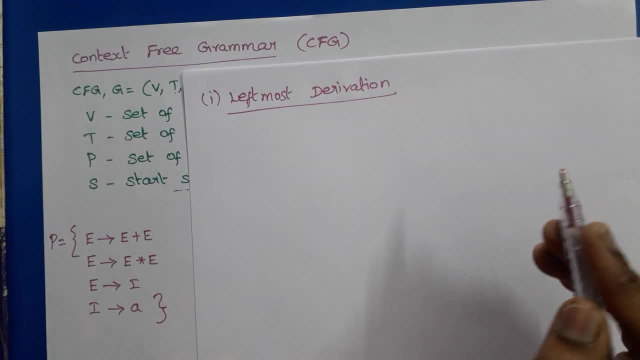 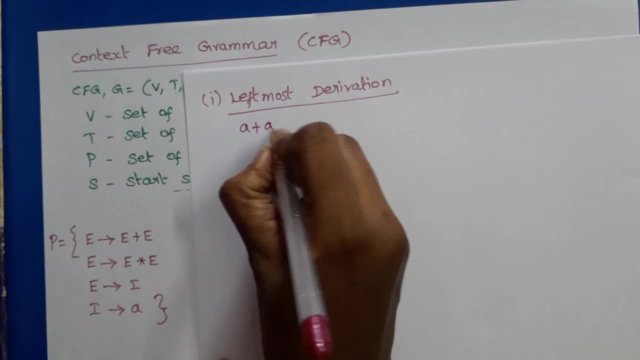 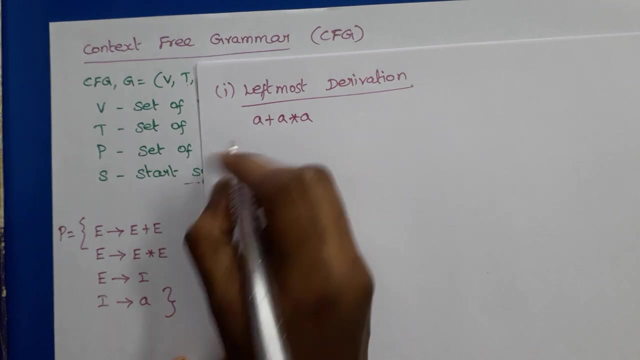 production bodies. so in right most derivation we replace right most variable by one of its production bodies. so let us derive a plus a star, a, the string, from this grammar. so every time we have to start with the start symbol of the grammar, so e. and one more thing: derivation means 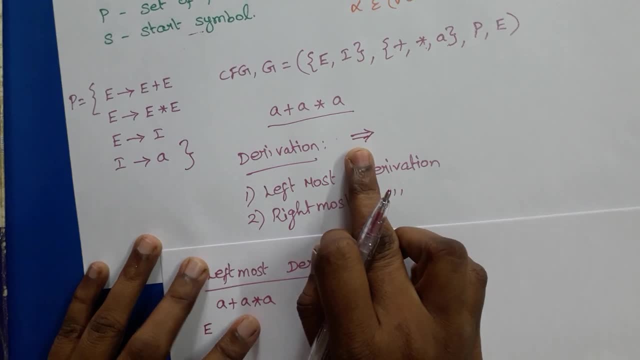 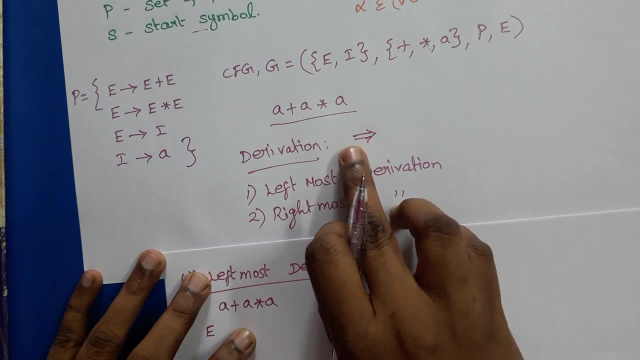 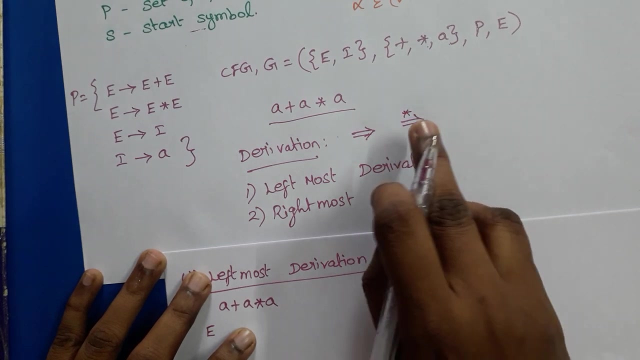 we need to use this symbol. this is the symbol for deriving- deriving a body of the production from the head of the production and it represents derivation in one step. so derivation symbol star: this is represents deriving in number of steps, more than one step. similarly for left most. 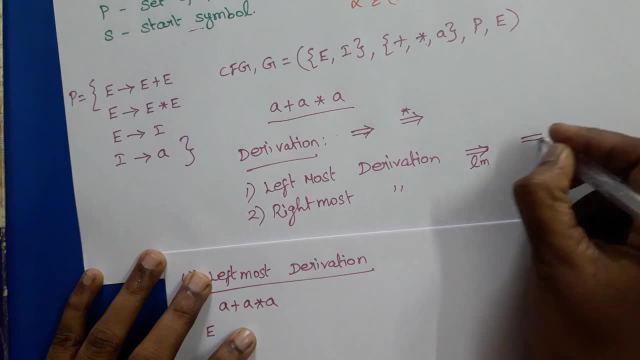 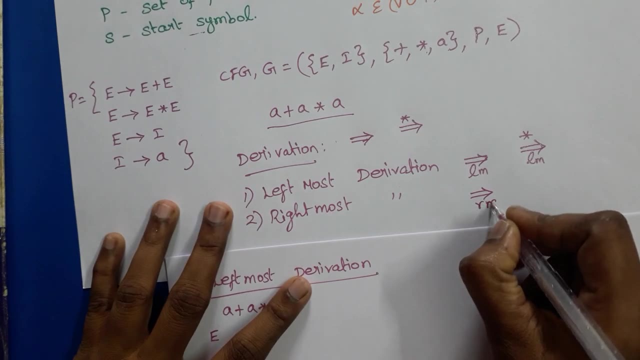 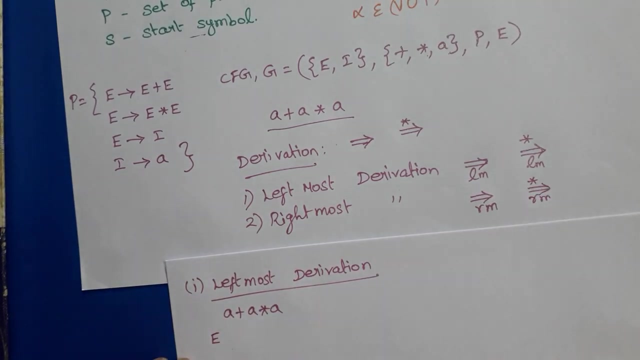 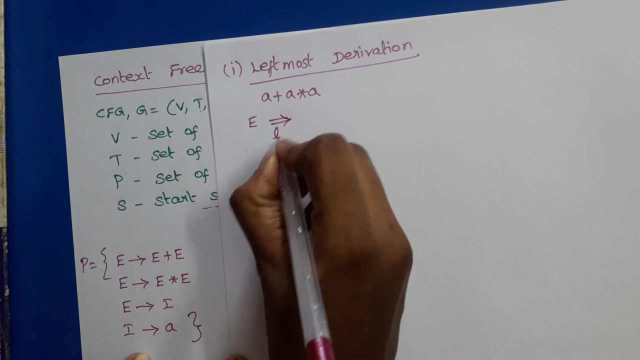 derivation means we have to use lm here and star lm represents more than one step. similarly, right most means r, m and right most derivation in one step. right most derivation in more than one step. so we have to use lm derivation symbol and lm here the meaning is: e derives e plus e in left most. 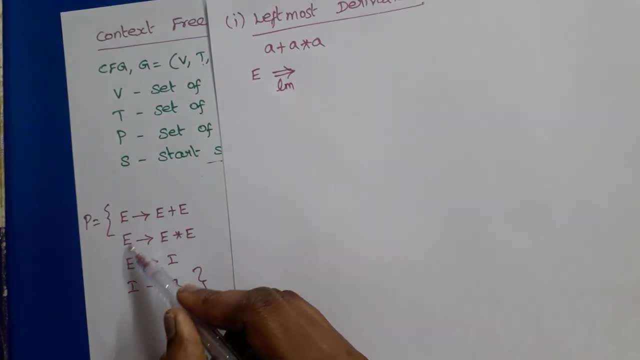 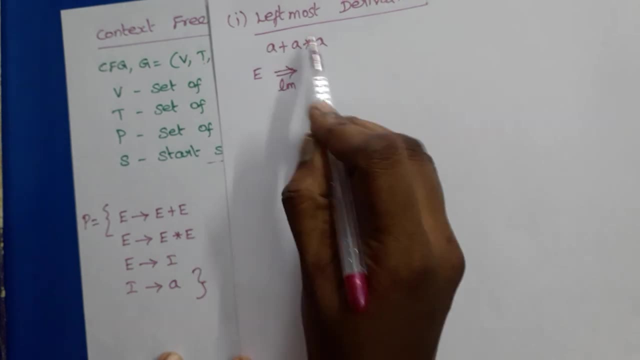 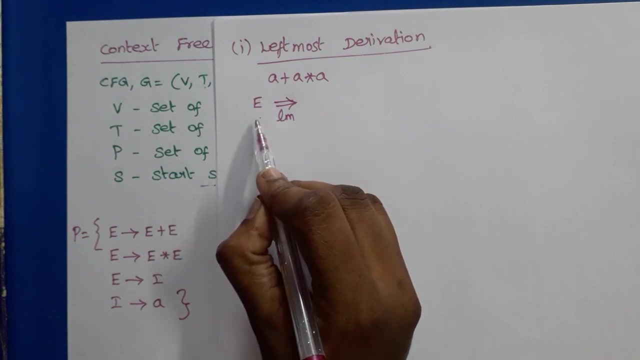 derivation here e has three productions right, e has three productions, e plus e, e, star e and i. we need to derive the string from the start symbol of the grammar in left, most derivation. so we have to consider the left most variable in the string. so here we have only one non- Terminal. 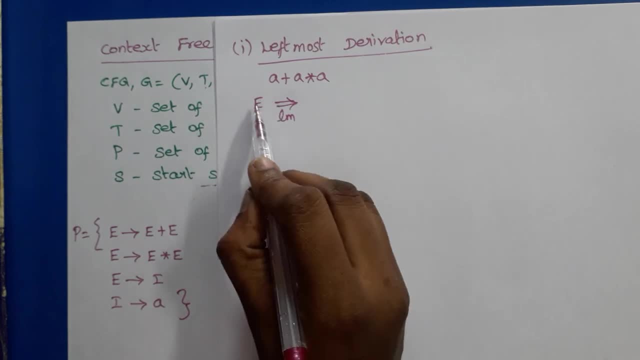 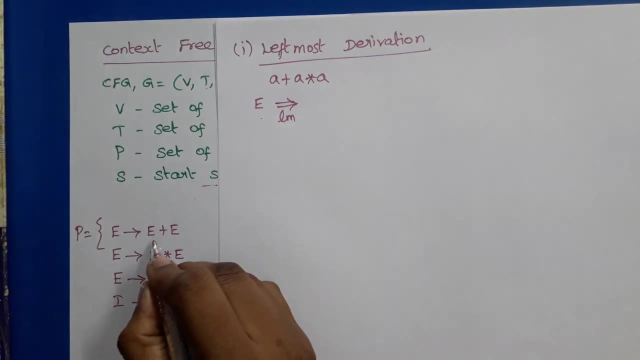 symbol only one variable, variable or non-Terminal. so this variable should be replaced by any one of the productions. here we need addition expression so we can use e plus e. so e can be expanded by using e plus e. or we can say that e derives in order to um, you know, to derived in order to plus by. you can use this as a derivative of a sum. so there are the terms, there are the terms c, a. here we need um god, um god. you have seen this definition. right now, men, also wasting your zeal, you are wasting your time, eraren. we have also how to principe this as well, so you probably have a text which is, In which case, black and white values. 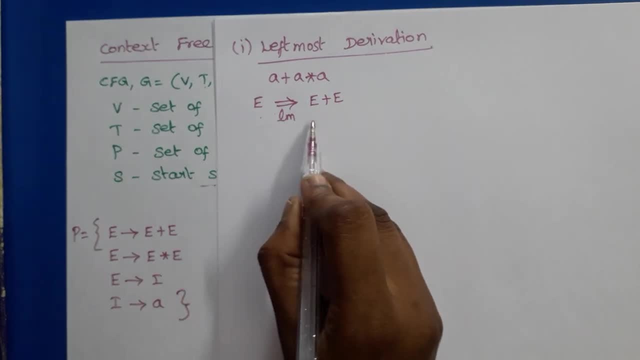 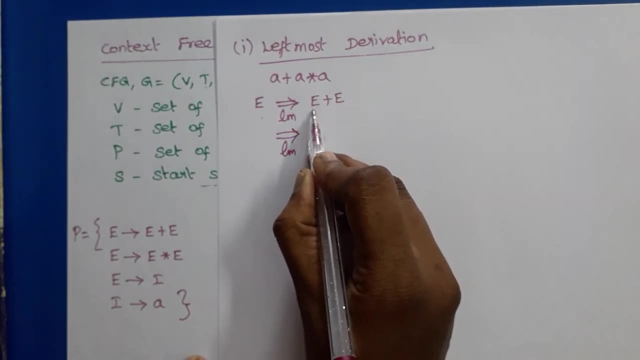 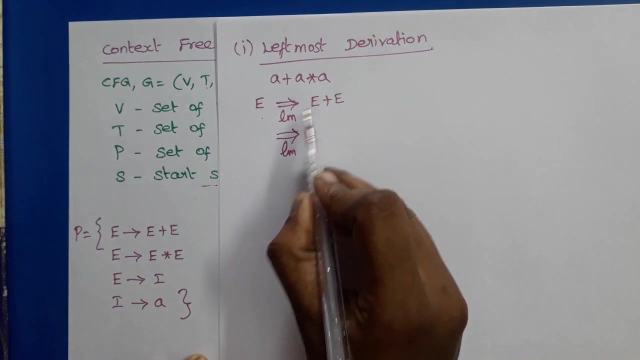 or we can say that e derives e plus e in leftmost derivation method. then in the next step in this string the leftmost variable is e. so before plus we need a. so e should be replaced by one of its production bodies. here the suitable production is e, tends to i, because in the next 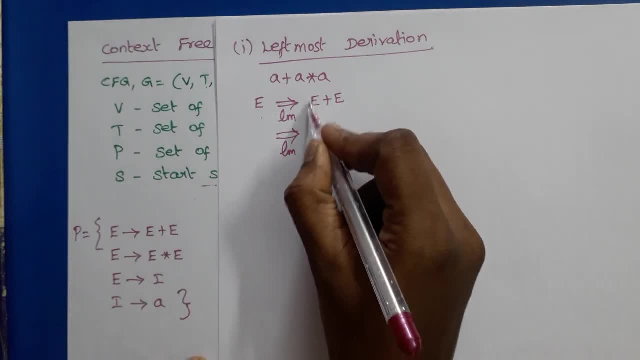 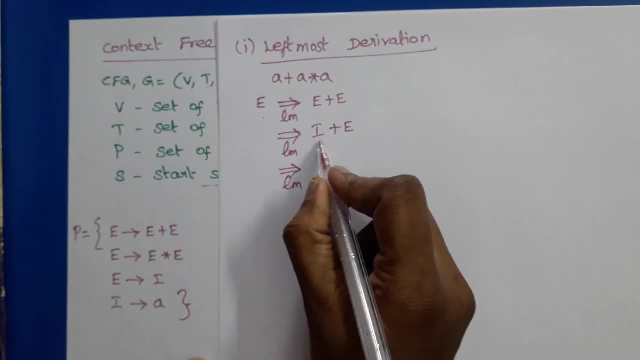 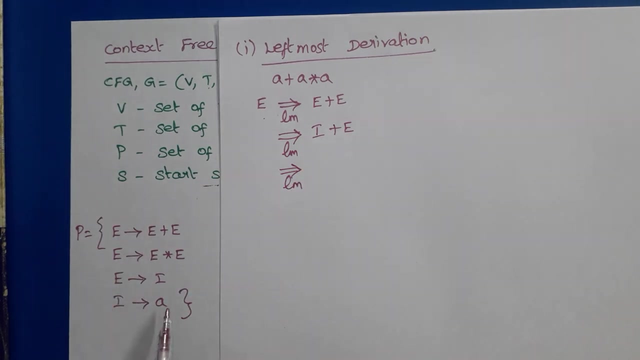 step we can replace. i tends to a, so e can be replaced by i. then in the next step, i is the leftmost non-terminal symbol, so that is replaced by a. so every time head of the production should be replaced by body of the production, so i can be replaced by a, now the leftmost non-terminal. 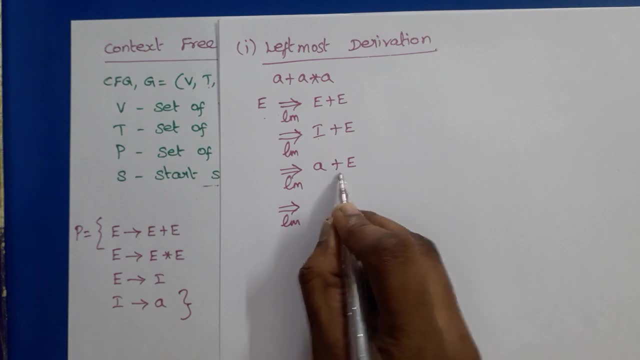 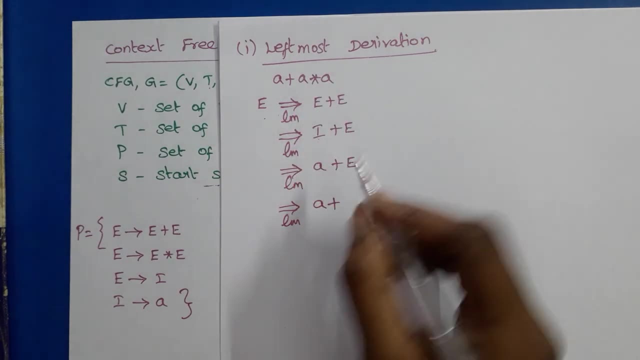 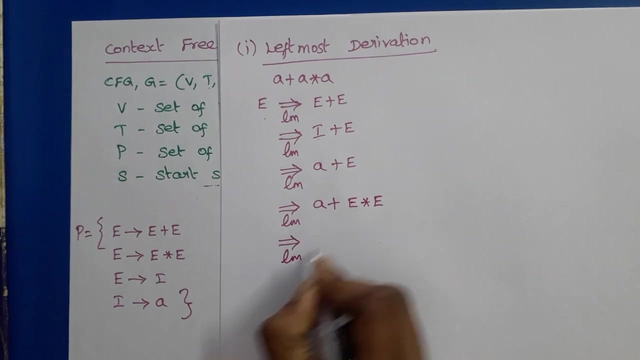 symbol is e, because these are. these two are the terminal symbols, so the leftmost variable is e. so this e must be replaced by here, we need a star a. so e must be replaced by e star e. then in the next step, this e must be replaced by here we need a. so 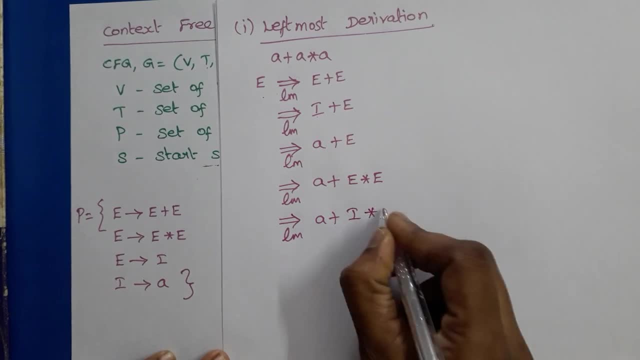 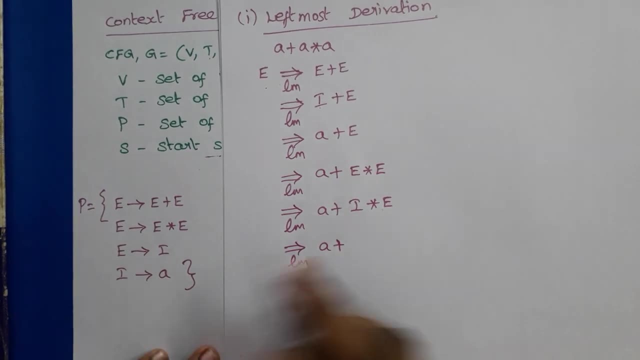 this e must be replaced by i. then in the next step, i must be replaced by a. then now the leftmost non-terminal symbol is a e, so this e should be replaced by i again, the leftmost non-terminal symbol is i. i has only one production, so we need to replace i by a, so we 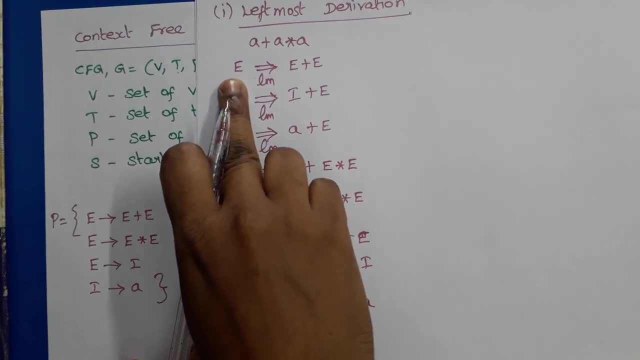 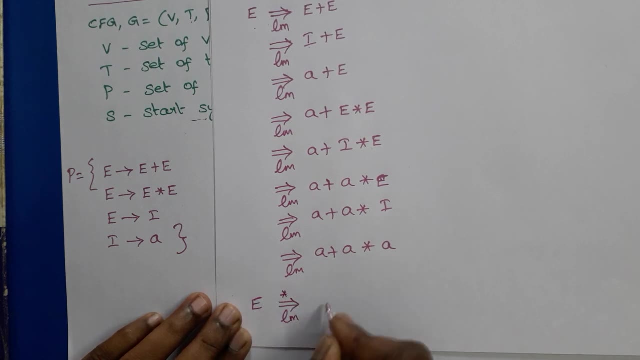 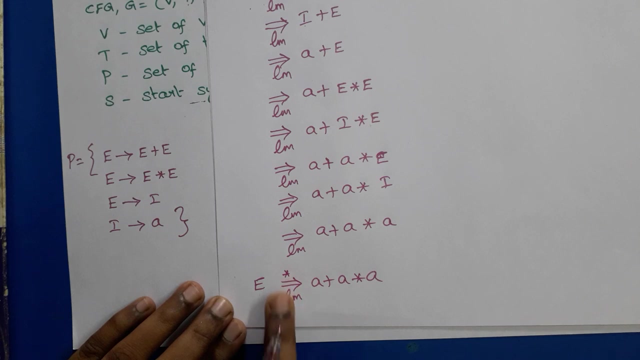 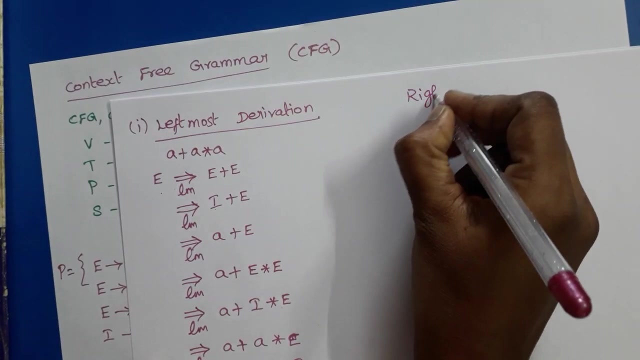 have derived a plus a star a from e in leftmost derivation method. we can also write e derived as a plus a star a in left most derivation. more than one step in more than one step. so now we will derive the same string using rightmost derivation, so rightmost derivation method. 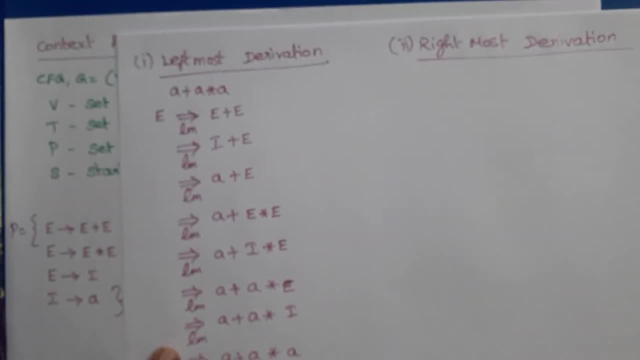 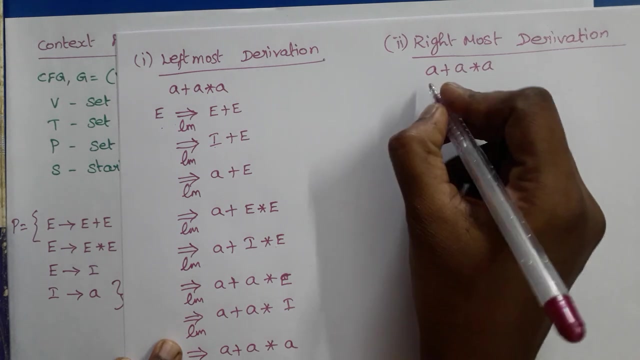 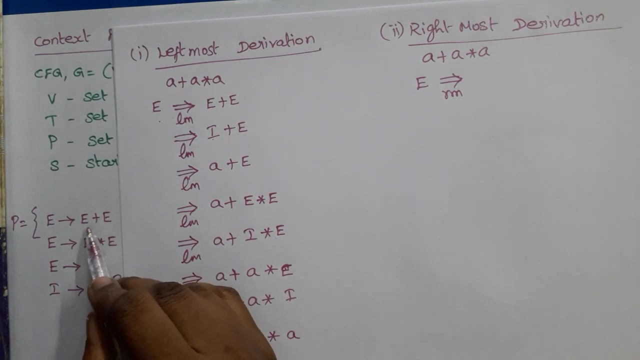 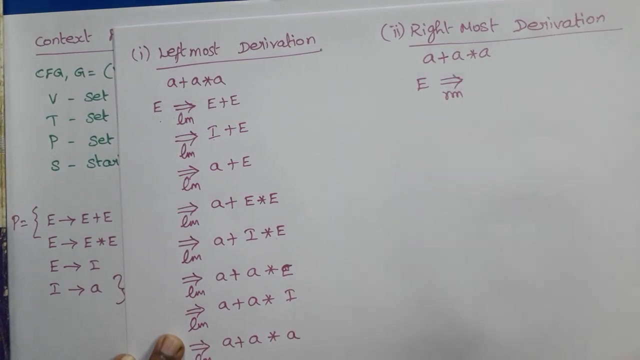 so here- here also we have- we are going to derive a plus a star a, but by using rightmost derivation method. so anyway, we have to start with the start symbol of the grammar, and here we need to write rightmost derivation so e can be expanded by using three productions. here also we need the same same string. 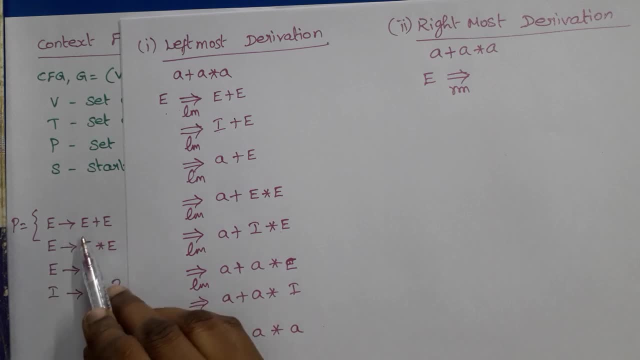 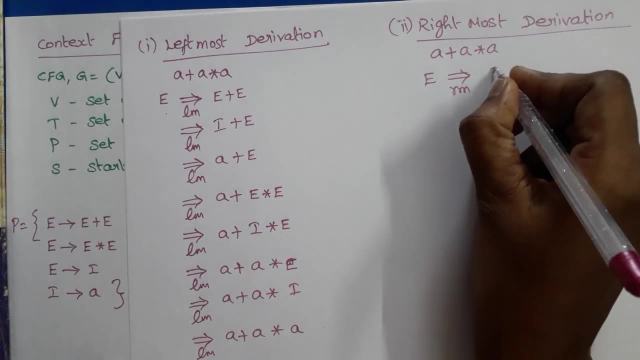 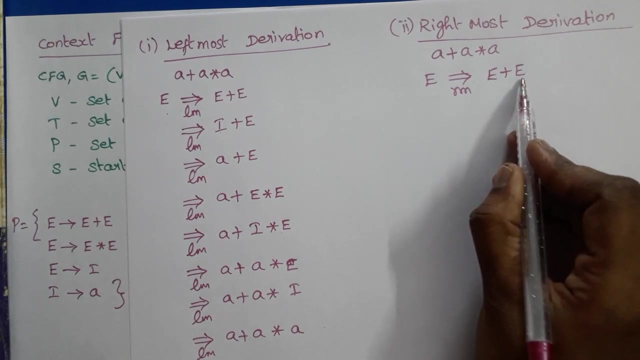 so e can be expanded by using e plus e, because here the rightmost variable is e, only so e. e can be expanded by using e plus e. now in the string the rightmost variable is the final e, so this must be replaced by one of its production bodies, so e. 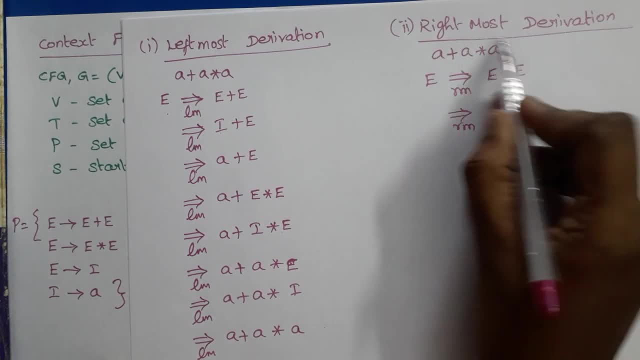 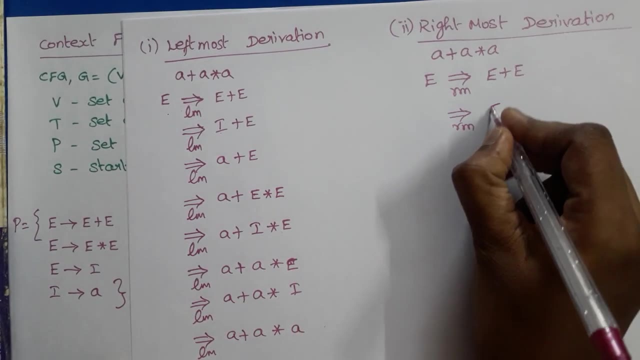 here after plus we need multiplication expression. so this e must be replaced by e star e. then only we can derive the string from the start symbol of the grammar. so e star e. now the rightmost non-transparent economic equation is e star e. so here we need to write rightmost derivation. 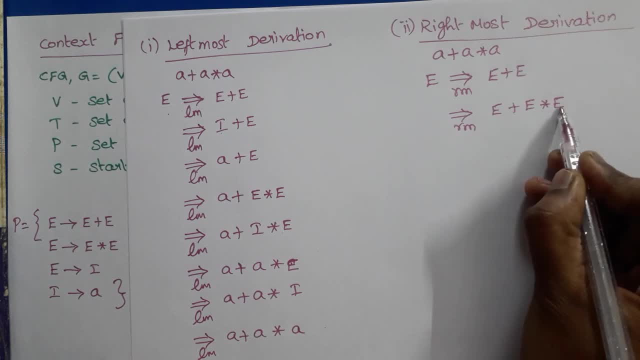 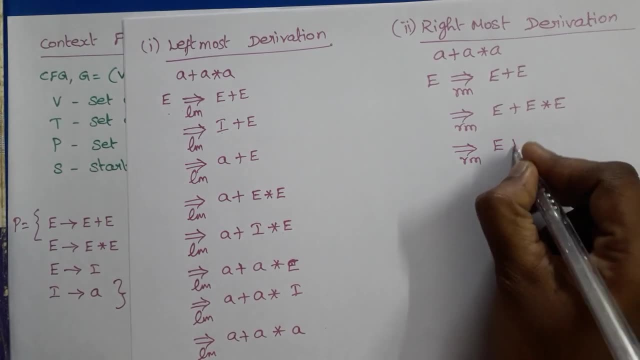 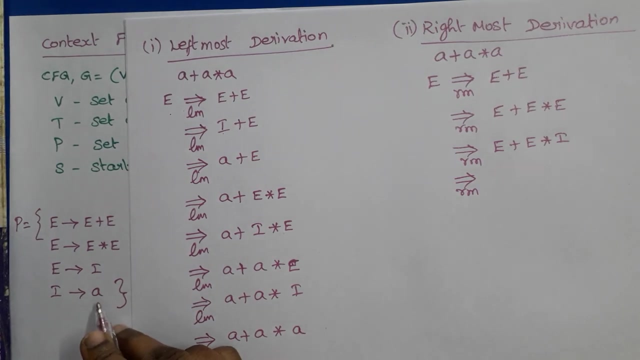 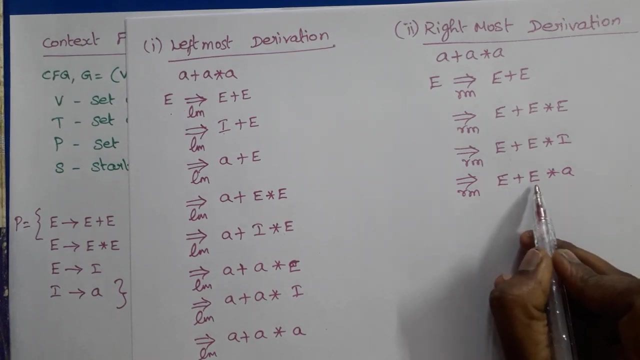 terminal symbol in this string is this: e. so this must be replaced by i in one step, and that i should be replaced by a. so e plus e star i, then the rightmost variable is i. i should be replaced by a. then, in this step, the rightmost variable is this: e the symbol middle symbol e. 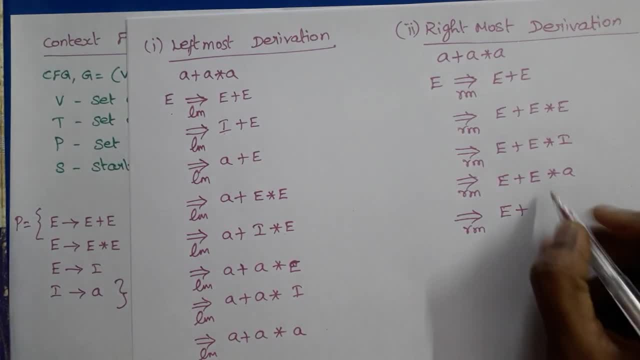 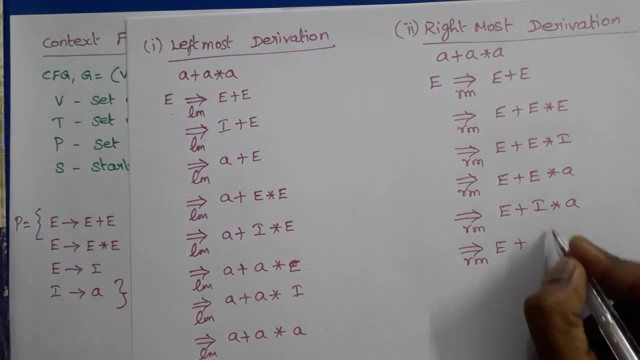 so e plus e should be replaced by i. then in the next step, i is the rightmost variable, so that must be replaced by a. then in this step, the rightmost variable is e. from the right end the first variable is e, so this e should be replaced by i. 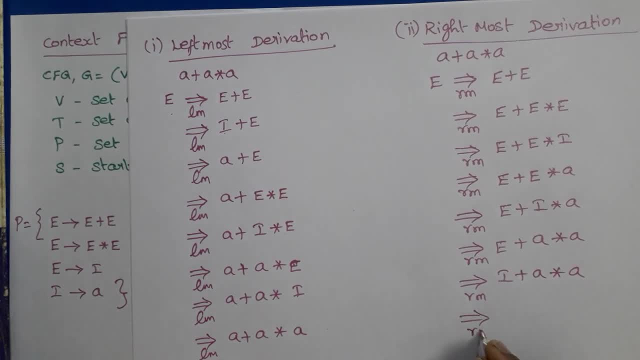 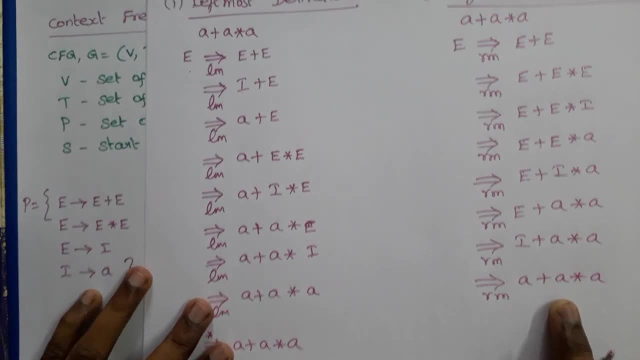 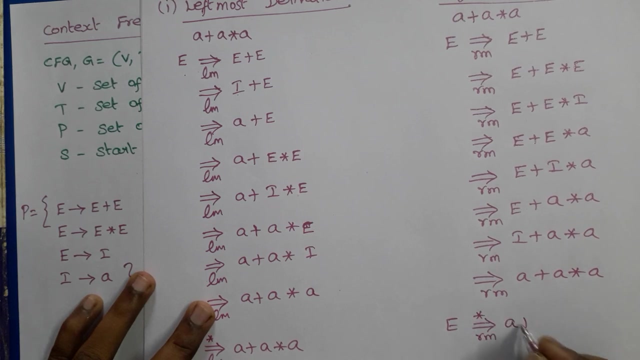 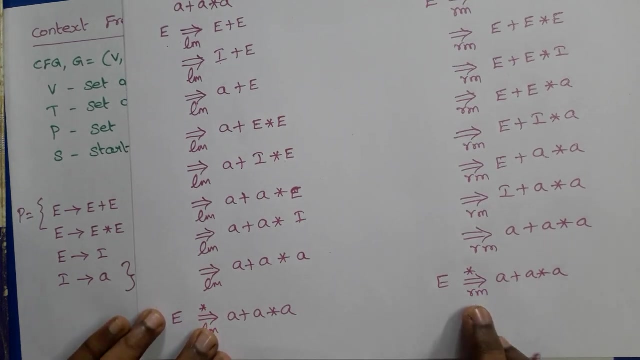 so then i must be replaced by a. so here we have derived the string from the start symbol of the grammar using rightmost derivation. we can also write like this at the end: after deriving this, you can write like this: e derives a plus a star, a in rightmost derivation, in more than: 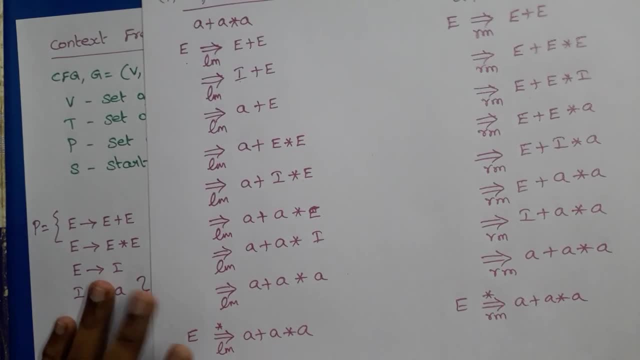 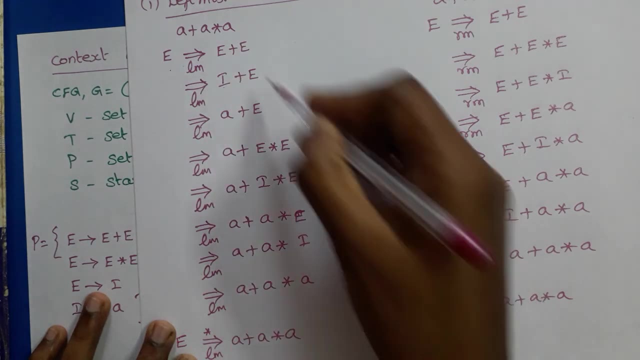 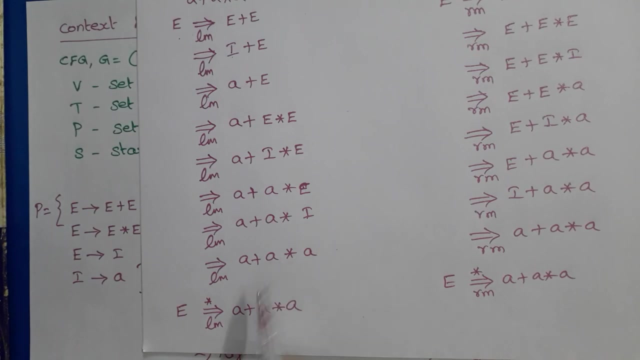 some number of steps by following some number of steps. so now these are the intermediate steps. these intermediate strings are called as sentential forms, so it may have both the terminals and non-terminals, okay, but the final string is all the terminal symbols. so now we can. 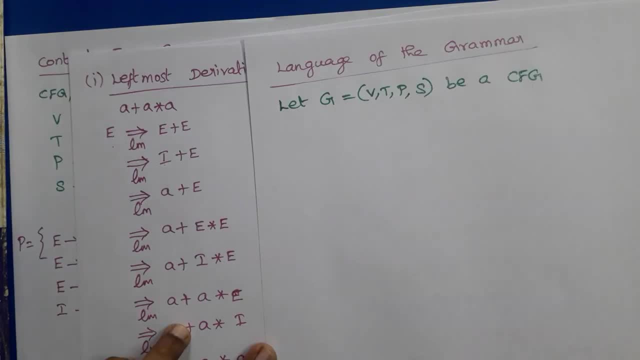 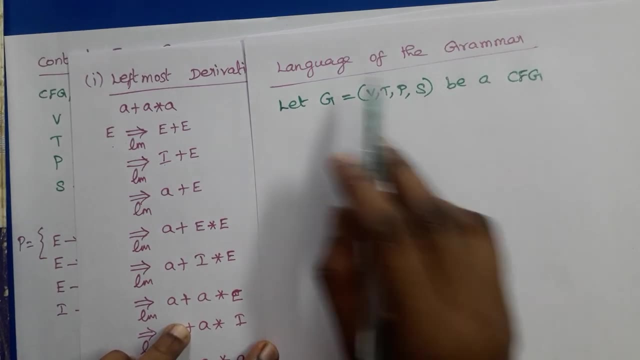 write the language of the grammar. so the language of the grammar let g is equal to vtps, vr, context free grammar. then the language of the grammar is written as l of g. l of g represents language of the grammar is equal to set of strings w. okay, the language of the grammar is set of. 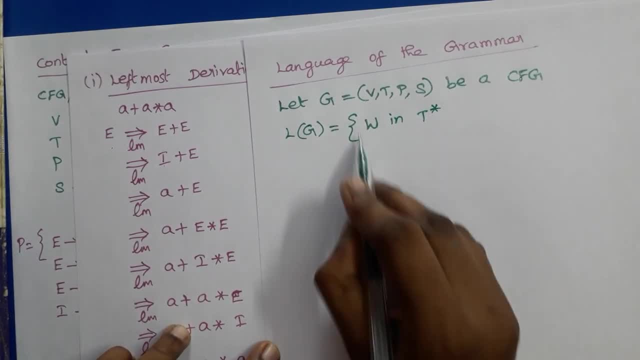 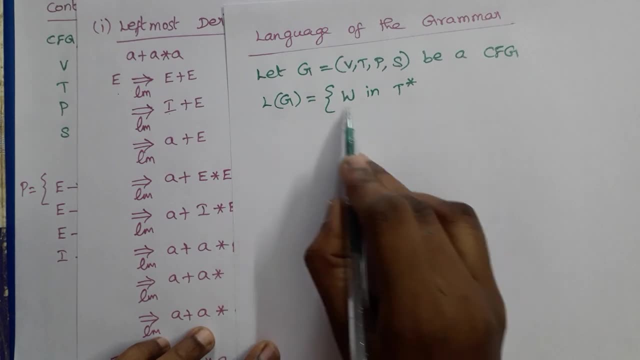 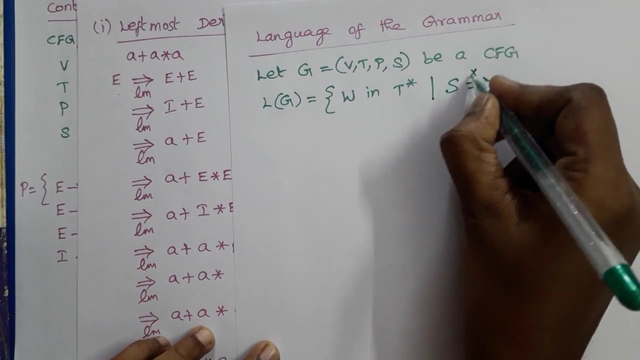 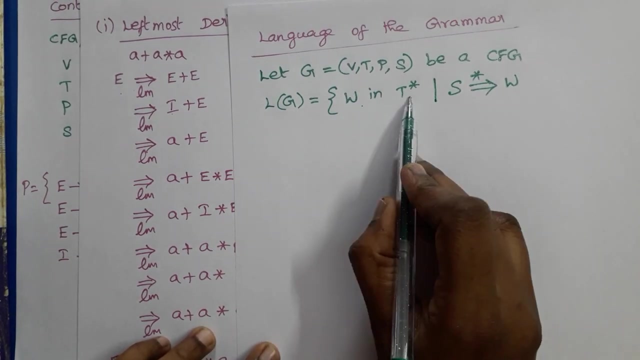 strings w in t star the meaning is terminal string. all the symbols must be terminal symbols. so l of g is equal to set of strings in t star, such that the start symbol of the grammar yes derives this string w in some number of steps. okay, so l of g is equal to set of strings w in. 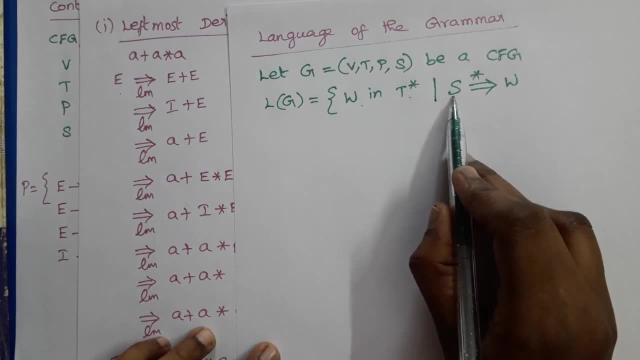 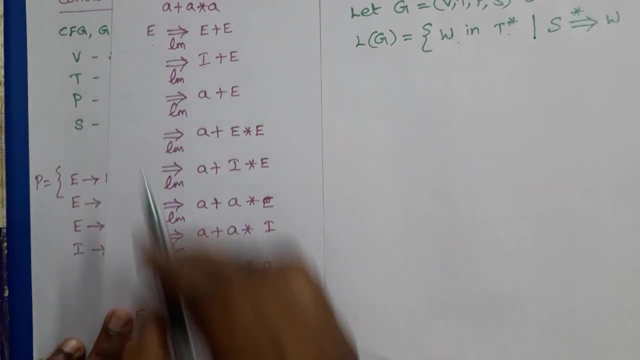 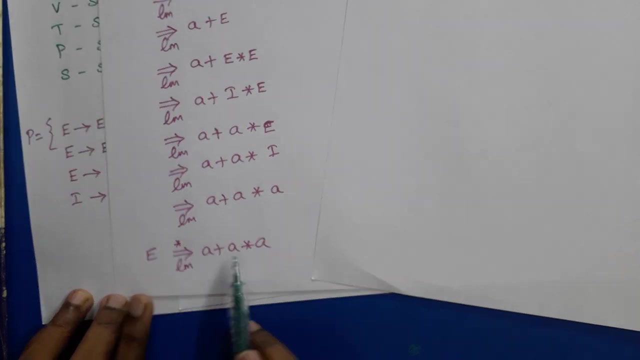 t star, such that start symbol of the grammar must derive this w in some number of steps. so here this start symbol of the grammar e derives. start symbol of the grammar e derives a plus a star a in some number of steps. so we can say that a plus a star a is a. 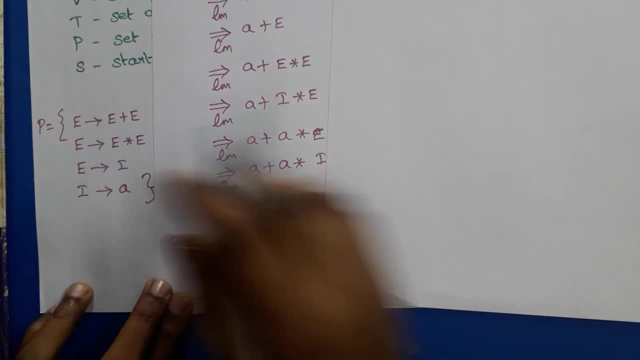 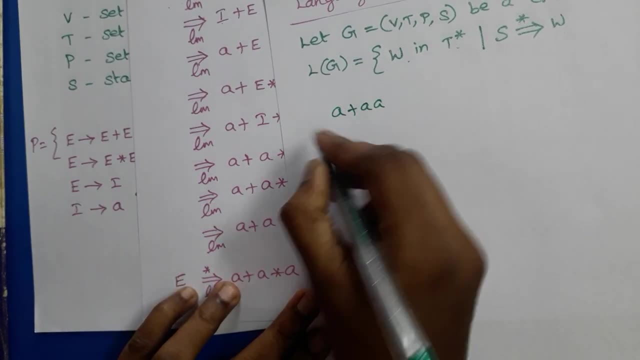 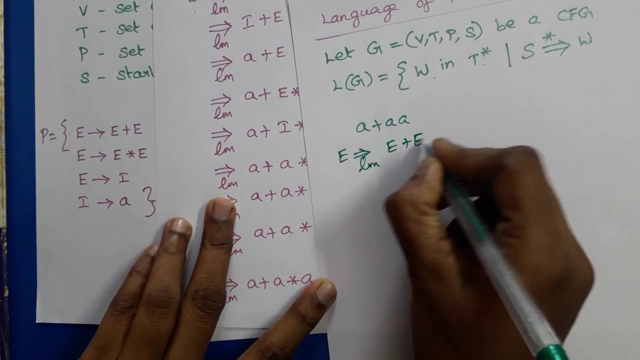 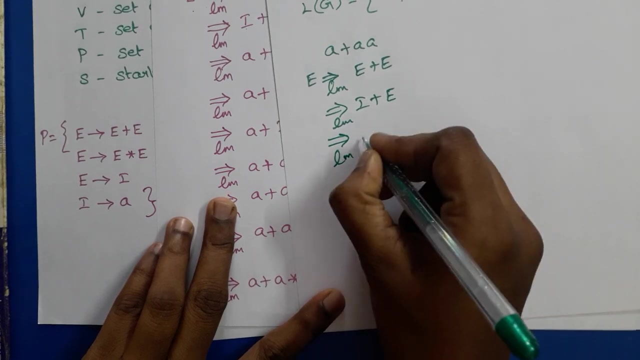 string a of this string generated by this grammar, okay, but we cannot say a plus a. a is a string derived from this grammar, right? because we can try to derive the string e derives in leftmost derivation e plus e. then e can be replaced by i, i can be replaced by a and this e can be replaced by. 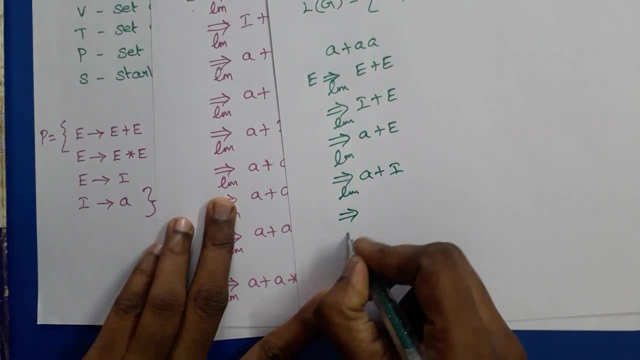 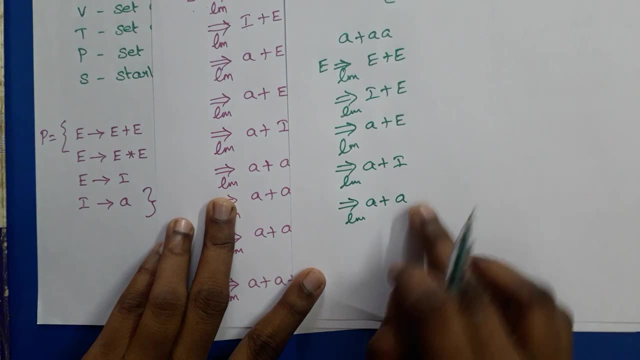 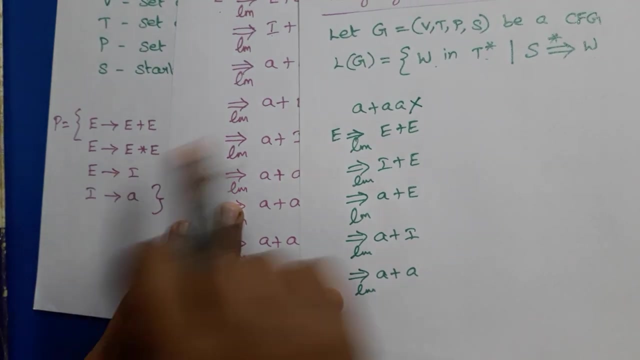 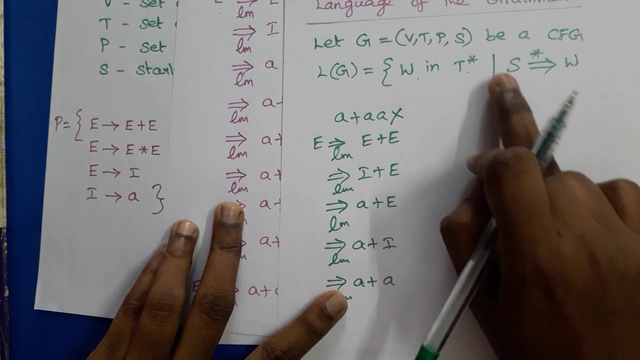 i and then a, but we didn't derive the last symbol. right, we can't derive this a by this grammar, so this string is not belonging to this particular grammar. okay, so language means set of strings, set of terminal strings, such that, yes, derives start symbol of the grammar, derives that string. 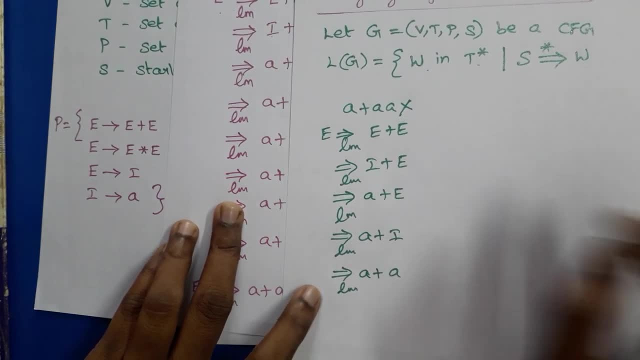 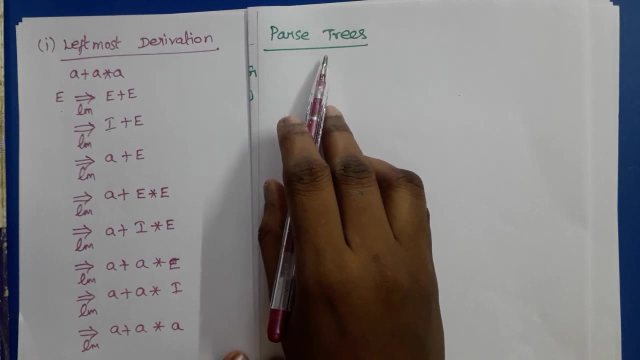 in some number of steps. it may be leftmost derivation of that string. in some number of steps, derivation or rightmost derivation, we can use any, any step, any method. the next one is parse trees. parse trees are the tree representation of derivation. tree representation of derivation is called as parse tree, that is, we can also draw tree like structure for the for deriving the. 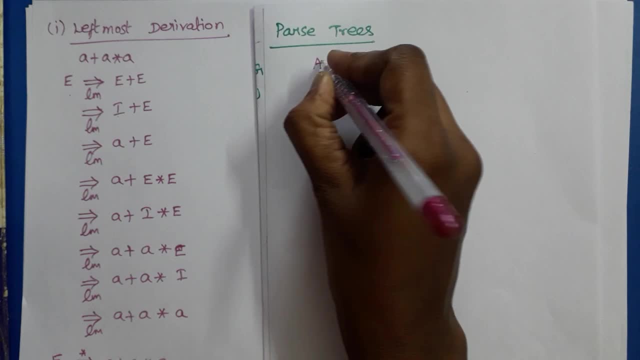 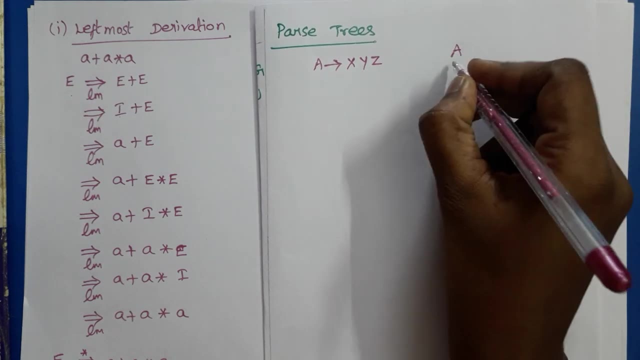 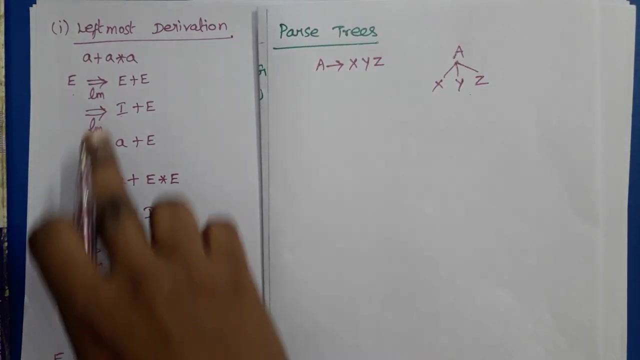 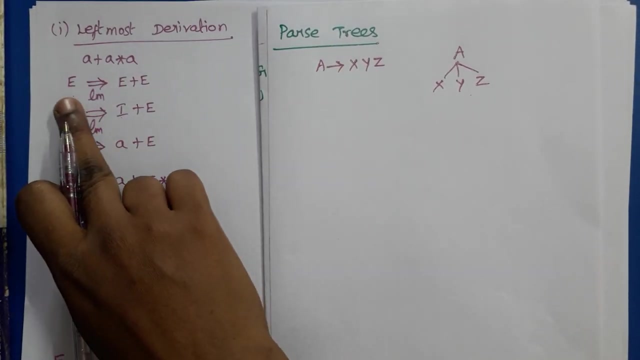 string. so, for example, if the production is a tends to x, y z, then in a parse tree the parent a has three children, x, y, z. we need to draw like this, we have to expand like this so we can derive the string a plus a star a from the start symbol of the grammar using parse tree. okay, so here. 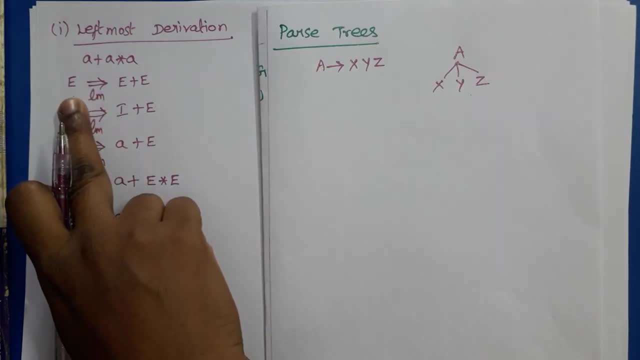 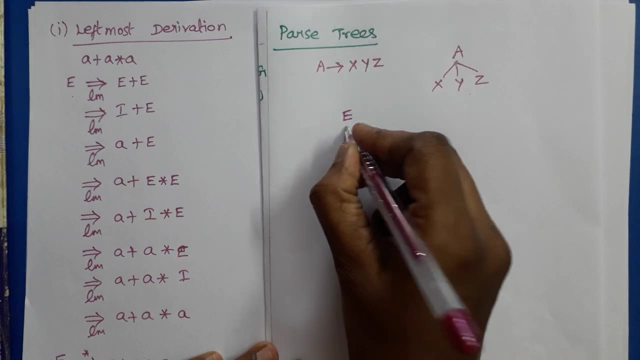 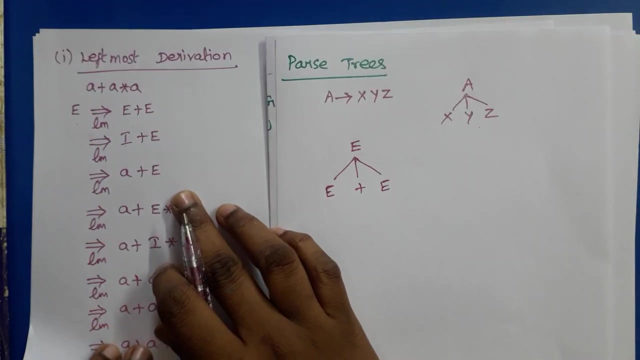 the root of the parse tree is always the start symbol of the grammar. so a e and e derives e plus e right. so that can be expanded like this. so by using either we can follow the productions. so the grammar is: e tends to e plus e, e tends to e star. 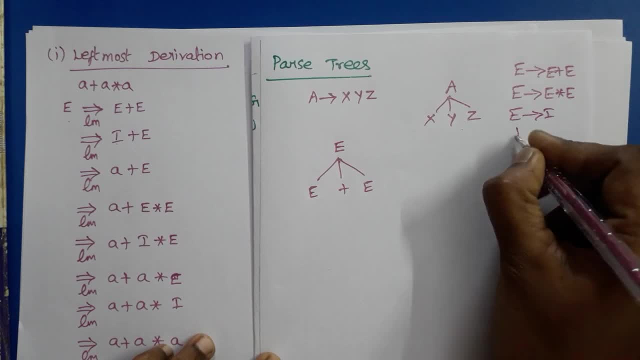 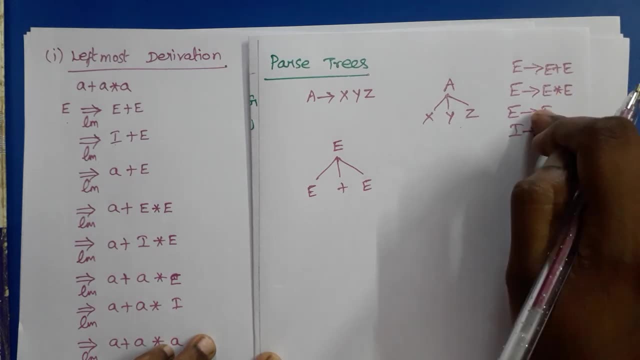 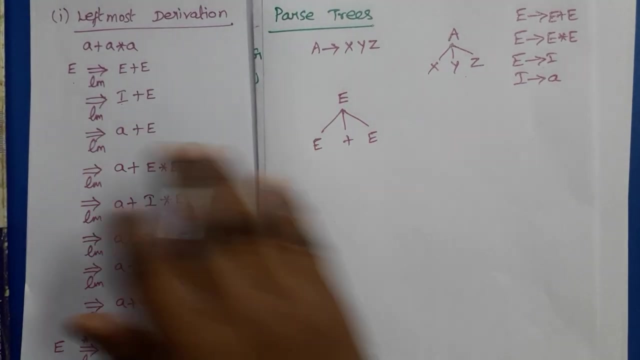 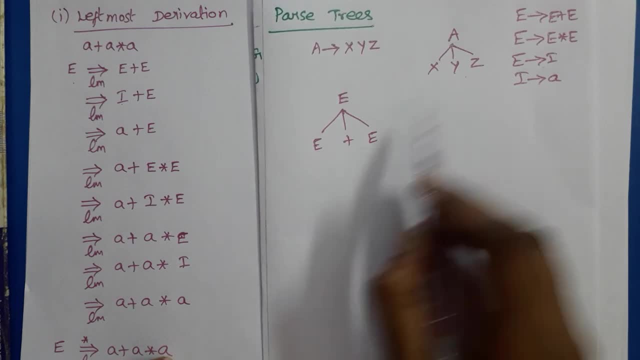 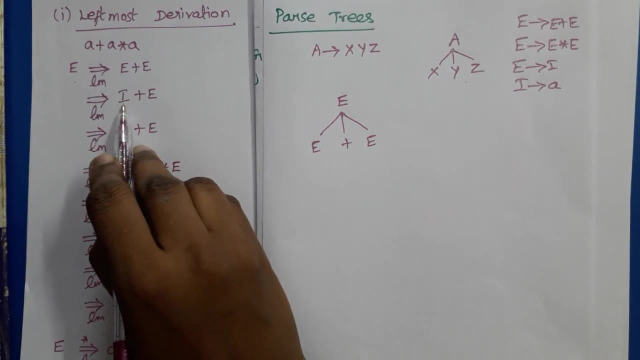 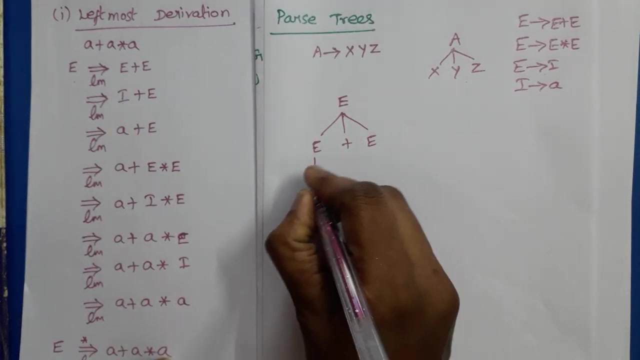 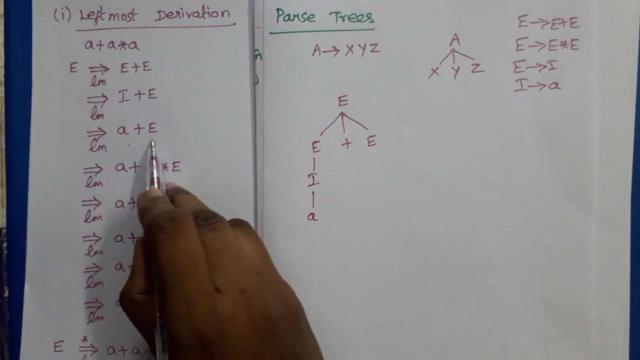 so e has three children, e plus e, or we can take this production for expanding like this. then e. this e is replaced by i. there is no change in plus and e okay, so e is replaced by i. then in the next step, i is replaced by a. the meaning is: i has one child, a. then in the next step, this e is replaced. 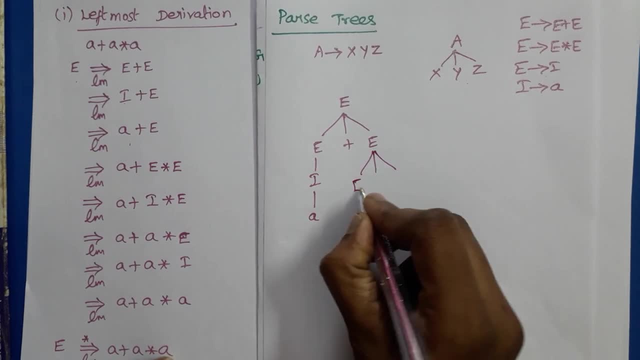 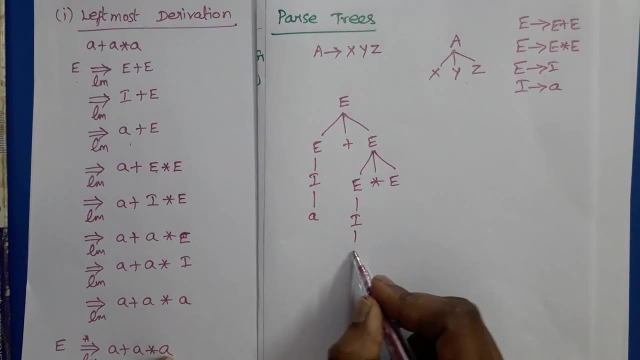 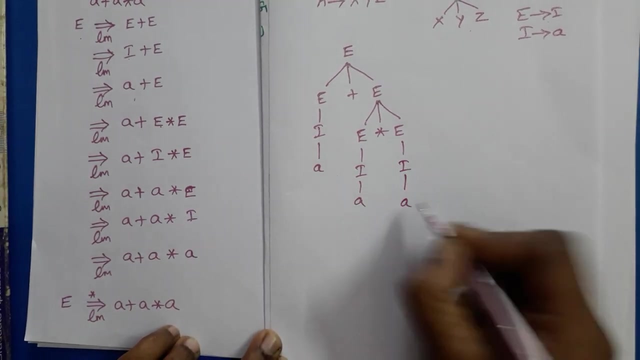 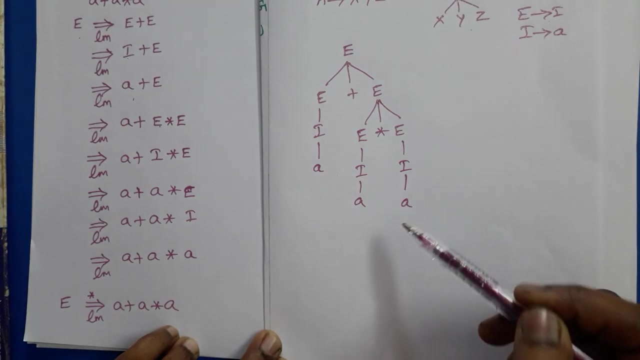 by e star e. so this e has three children: e, star e, and this e is replaced by i and the i is replaced by a. in the next step, e um e is replaced by i and i is replaced by a. so in the parse tree, interior nodes represent the variables and leaves represent the terminal symbols, or sometimes epsilon. epsilon. 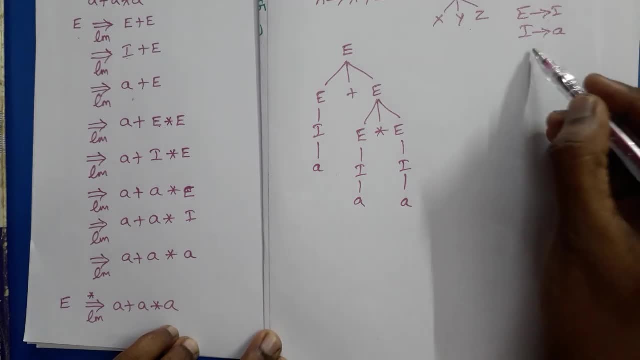 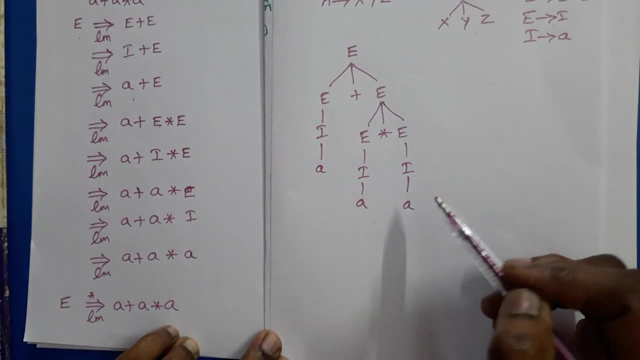 also we will use, suppose, if i tends to. epsilon is a production, i can also be replaced by epsilon. so the term leaves represent a. a leaves indicate either a terminal symbol or epsilon. and if we can candidate the leaves from the left end, uh, if we parse the three from a, traverse the three. if we traverse the tree, then we will. 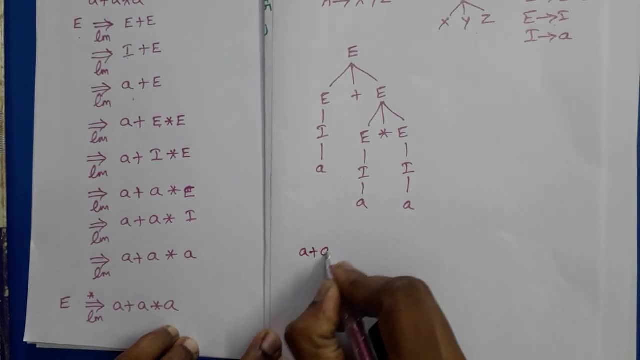 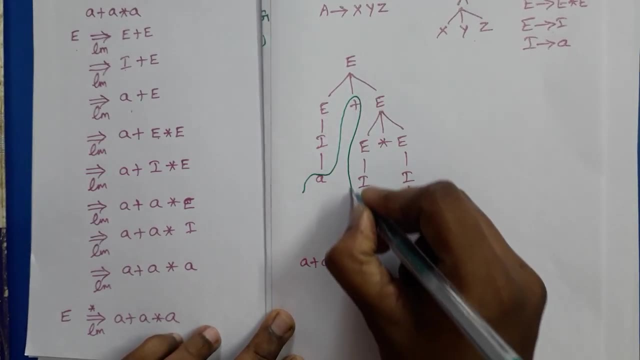 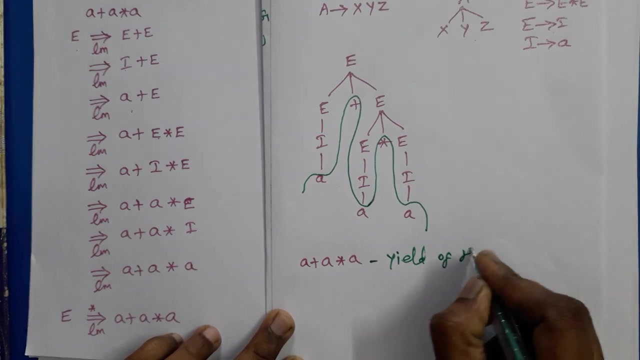 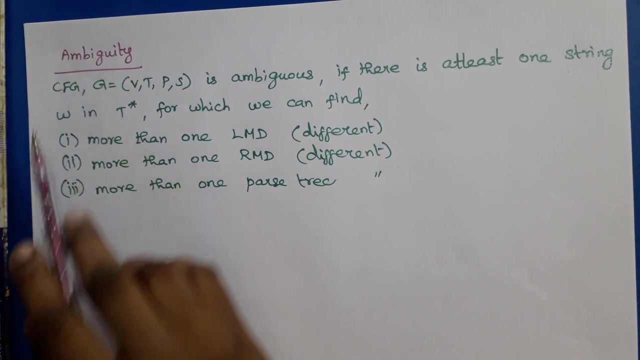 get the string a plus a star a right. if it travels this tree, we will get a plus a star a. so this is This is called as yield of the parse tree. Next one is ambiguity. a grammar a CFG G is equal to VT. PS is said to be ambiguous grammar. 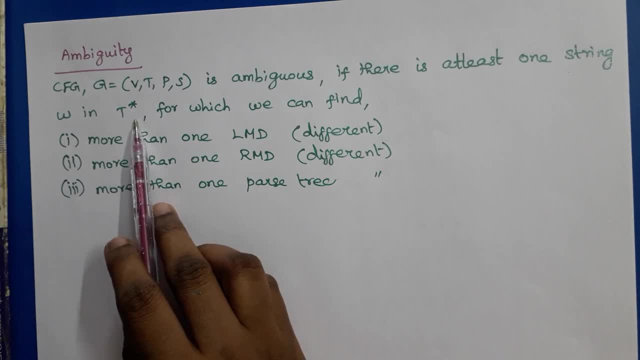 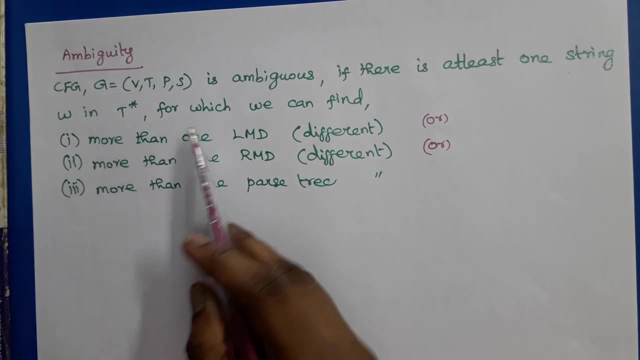 if there is, at least for one input, string W in T star, for which we can find more than one leftmost derivation, or more than one rightmost derivation, or more than one parse tree. Okay, so either if we can find two or more different leftmost derivation for one particular, 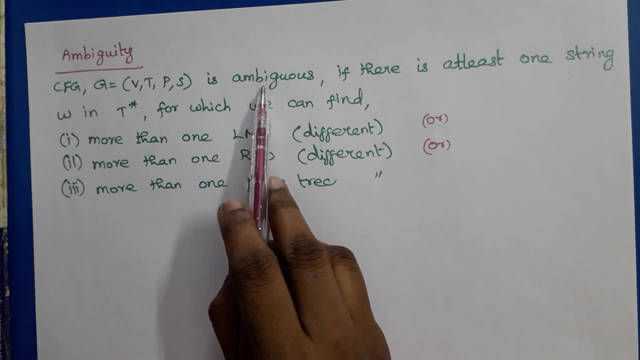 string of the context free grammar, then we can say that the context free grammar is ambiguous. or if we can find two or more different rightmost derivation for the same string means, we can also say the grammar is ambiguous. or if we can draw two different parse trees, two or 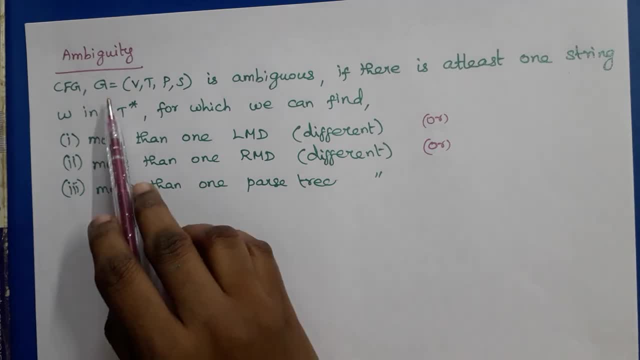 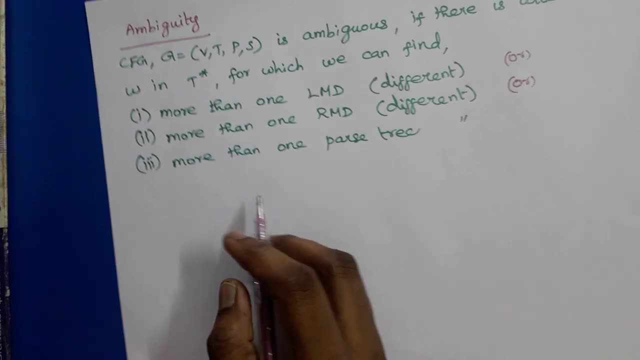 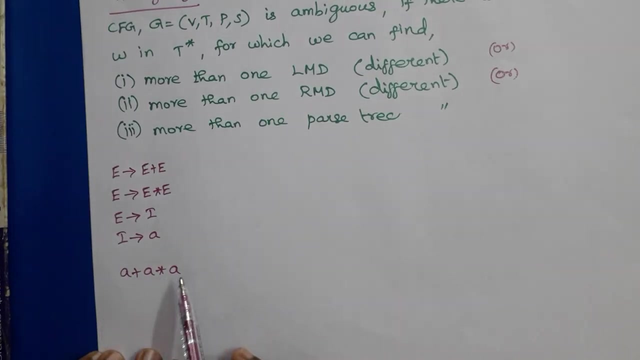 more different parse trees for the same string means we can say the given grammar is ambiguous. so now we will consider the same example and try to draw two different parse trees. so consider the same grammar and we are going to derive the string a plus a star a. 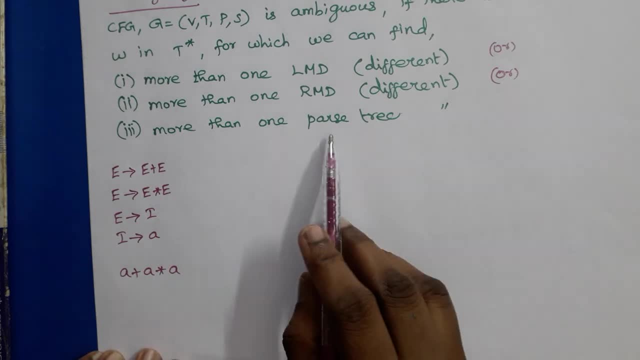 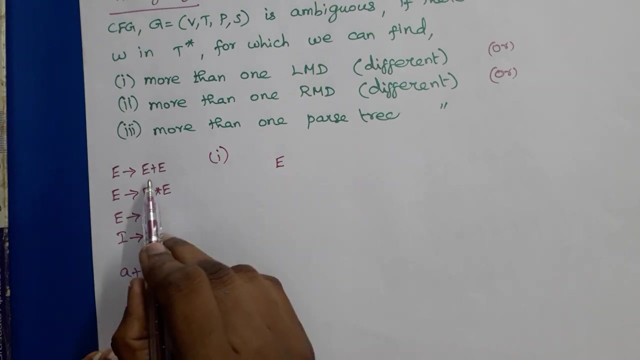 so in a, by drawing the parse tree, two different parse trees, so we can say that the given grammar is ambiguous. so here the root of the parse tree is start symbol of the grammar. so e. this is a first parse tree, so e. e can be expanded by using e plus e. 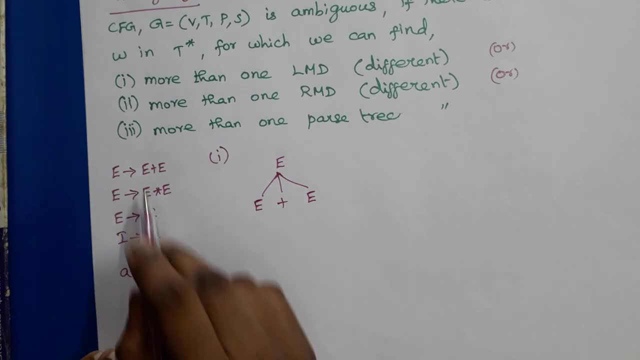 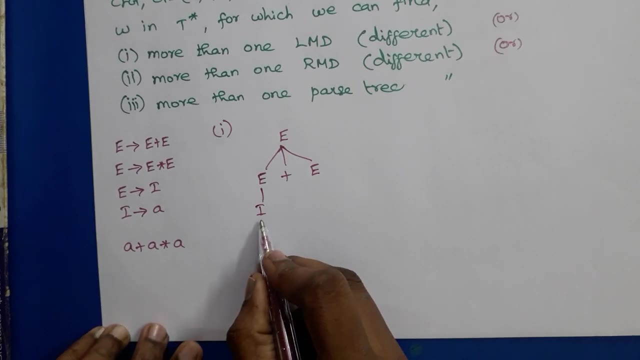 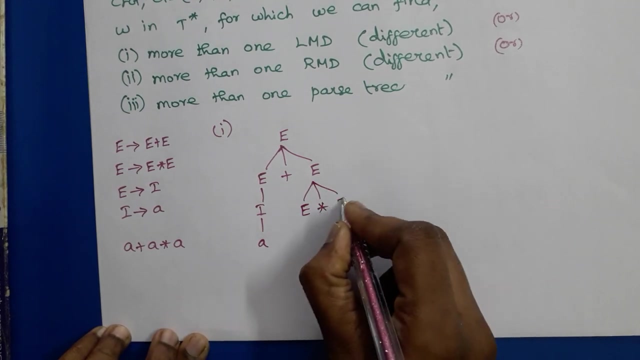 then this e before plus. we need a right. so e must be replaced by reduced to ai, and i can be replaced by a, and here this e can be replaced by e, star e. so by following this, by using this production, then e tends to i, so e can be expanded by using i. 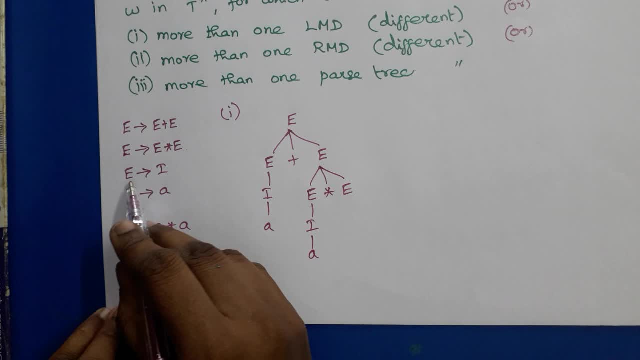 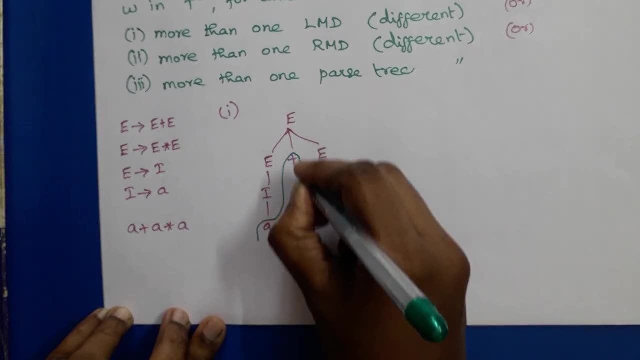 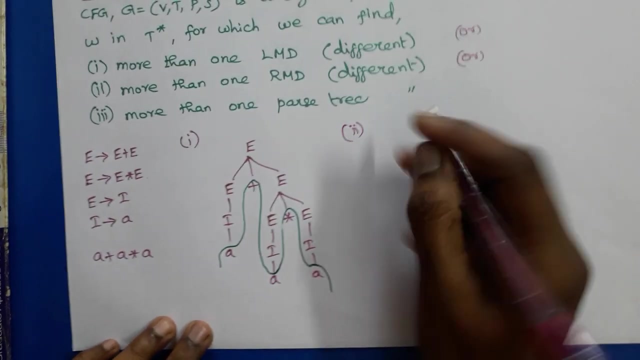 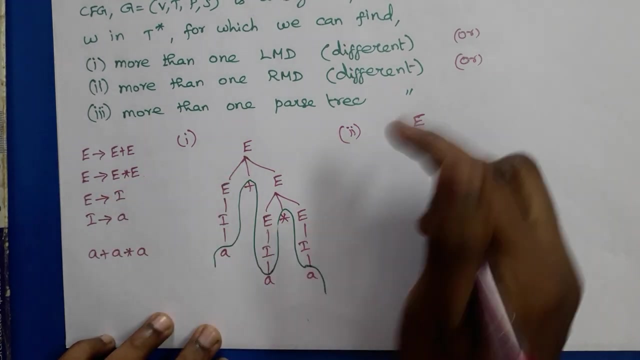 then i tends to a, so a, then this e can be i, then a. so if we concatenate this we get a plus a star a. we can try to construct another parse tree for the same. so e is a start symbol of the grammar. so here we can start with the second production: e, star e. 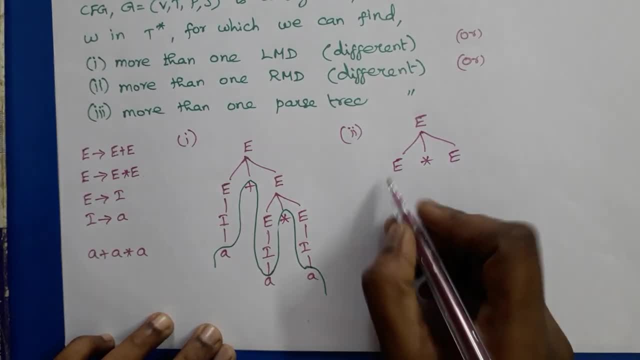 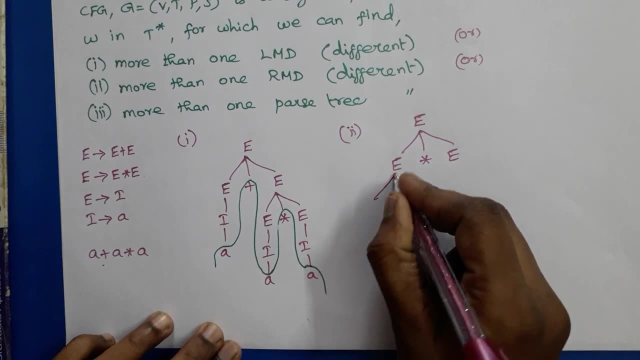 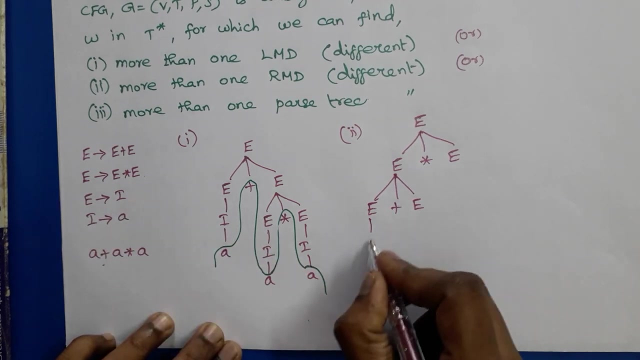 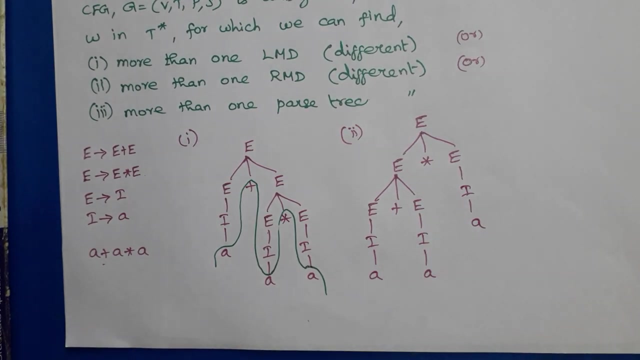 e star e, then before the star expression, we need a plus. so this e must be expanded by using the first production. so it has three children, e plus e, then this i sorry. e must be replaced by i and i can be replaced by a similarly this e and this e. so now we have got two different parse trees, right?